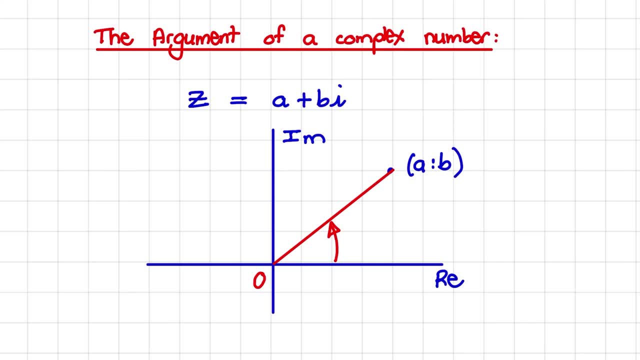 angle formed between the real axis and that line. So we have noted the argument here as theta, but it can also be noted as the arg of z, and that's the angle formed between the origin and the point on the complex plane. Now it's also important that we 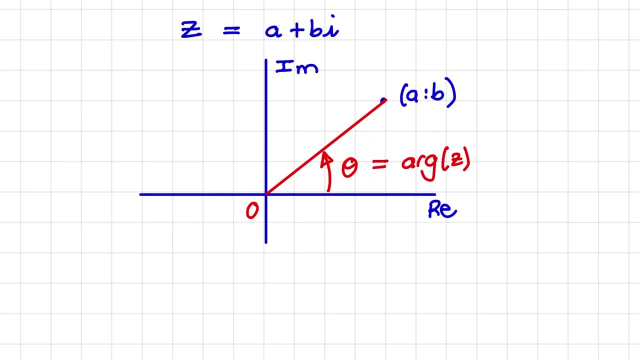 will not measure this angle in degrees, but we would rather measure it in radians. So the argument then is restricted between negative pi radians and positive pi radians. So that means I can go in an anti-clockwise direction up until I reach pi, or in a clockwise. 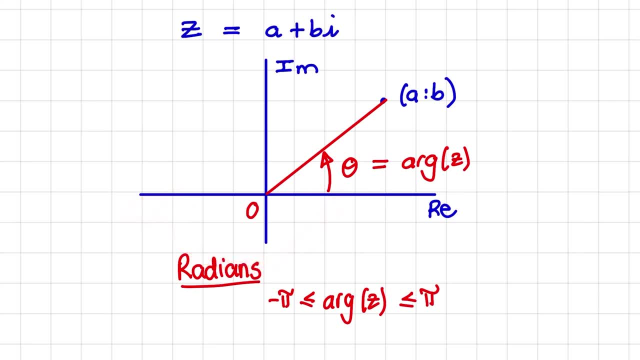 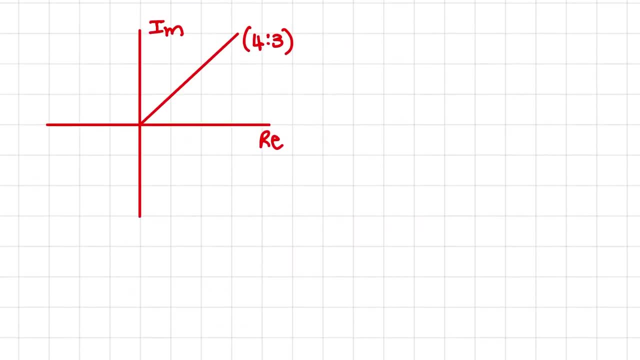 direction up until I reach negative pi. So that represents a full circle. Let us look at a few examples. In our first example we have a point in our first quadrant and we want to find the value of theta in terms of radians. So that's the argument of this complex number. So remember, I can create a. 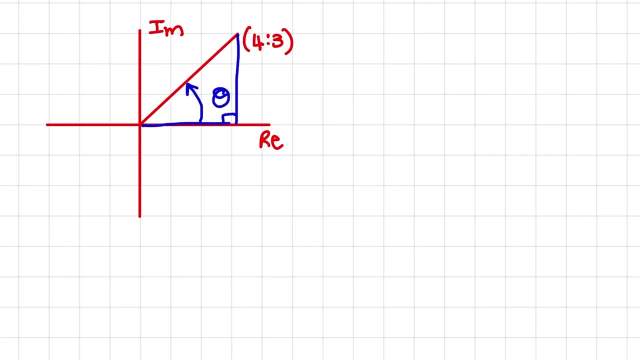 triangle, a right angled triangle, and what the four represents is the value adjacent to theta, and the three represents the value opposite, theta. Now, if I use trigonometry, I know that tan theta is equals to the opposite value divided by the adjacent value. So tan of theta would be equals to three. 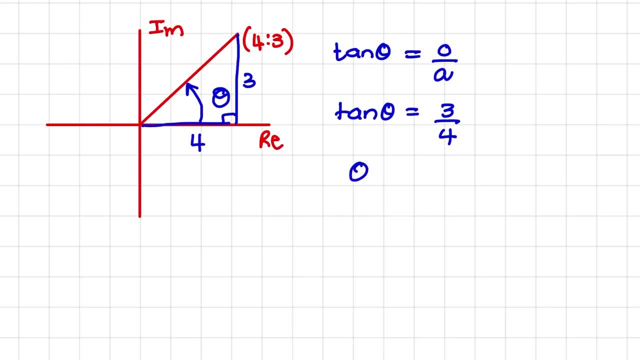 over four. Now, in order to solve for theta, I need to find the value of theta. So I need to find the value of theta. So, in order to solve for theta, I can use arc tan on my calculator. So my calculator, I put arc tan and I use three over four as my ratio and that will give me the value of theta. 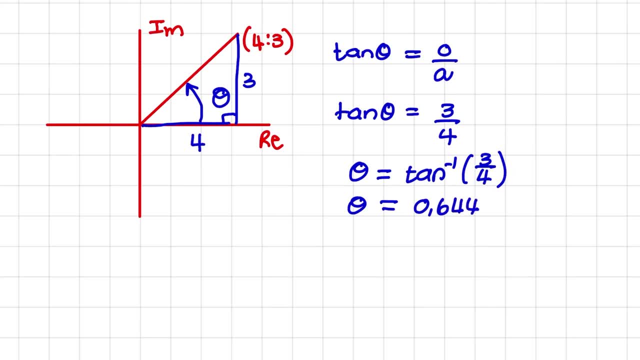 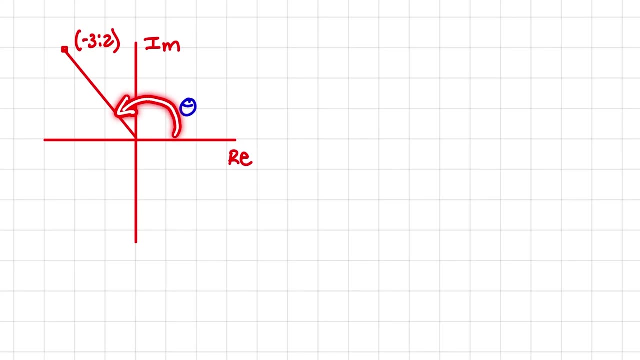 which is 0.644 radians. So remember to set your calculator to radians when we work with complex numbers. Let us look at another example in the second quadrant. So here we have the argument and we can see that the argument is past 90 degrees. So we find ourselves in the second. 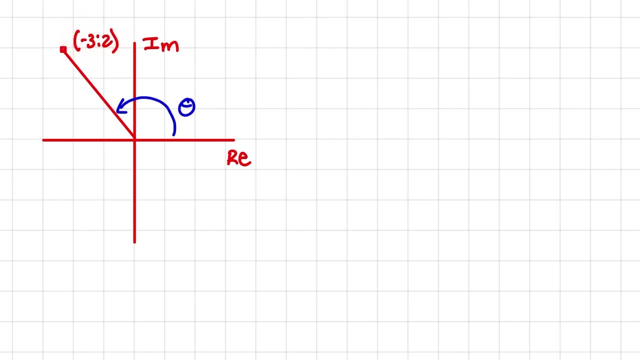 quadrant. Now we need to use a slightly different way of finding theta. So again, we will use tan, where the opposite value is two and the adjacent value is negative three. So we know that tan theta would be two over negative three. But to find theta we would say pi, which represents 180 degrees. 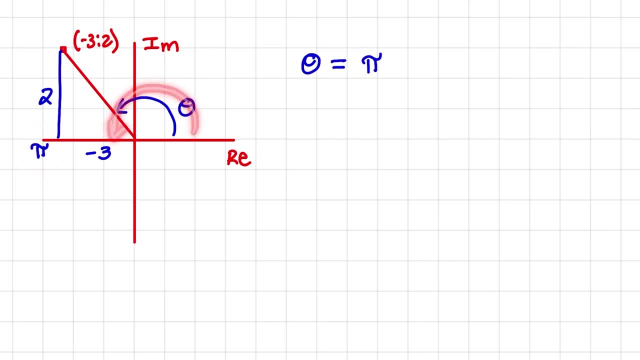 and we are going to go fully to 180 degrees and subtract this reference angle. So we would need to subtract that angle which is represented by tan. So we will use arc tan and the ratio that we would use is two over three. Notice, we are not concerned with the negative three, but we will use. 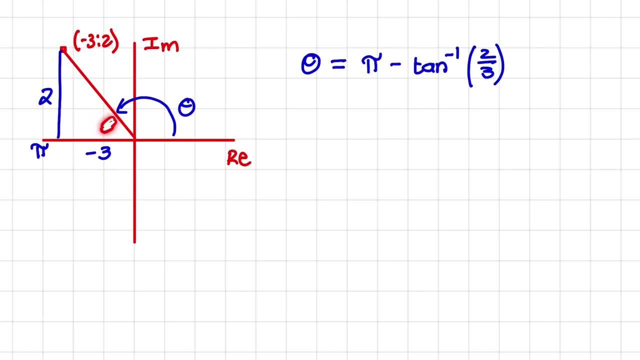 the absolute values in order to find this reference angle. So if I have pi minus this reference angle, then I have the size of theta, So that is equals to pi minus 0.588, and so on, And when I simplify I have 2.55 radians. Now let us look at a third example in the third quadrant. 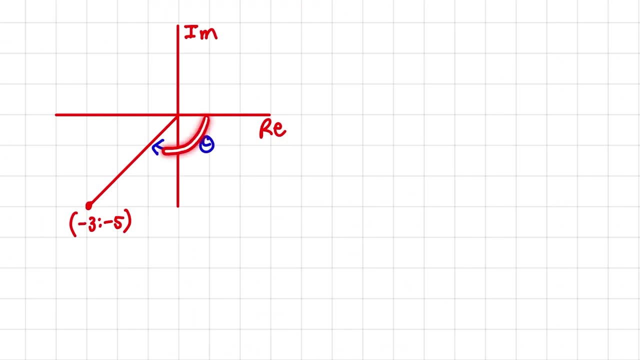 So in the third quadrant we will move in a clockwise direction from the real axis. So in the first two quadrants we moved in an anticlockwise direction from the real axis. So in the first two quadrants we moved in an anticlockwise direction. And now, to find the argument, we will move in a 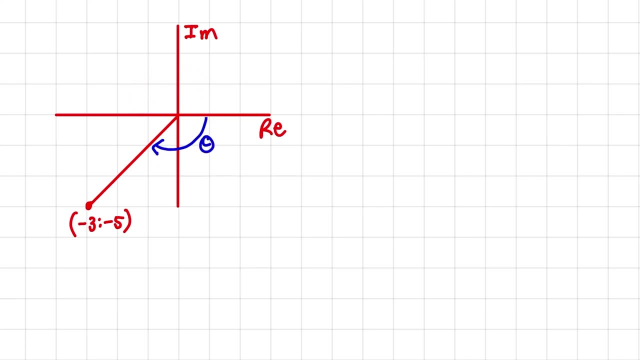 clockwise direction. So if I move all the way back to the real axis I would have moved negative pi radians or negative 180 degrees. And again, I can use a triangle to find this reference angle And that triangle and the length of that triangle would be minus three. 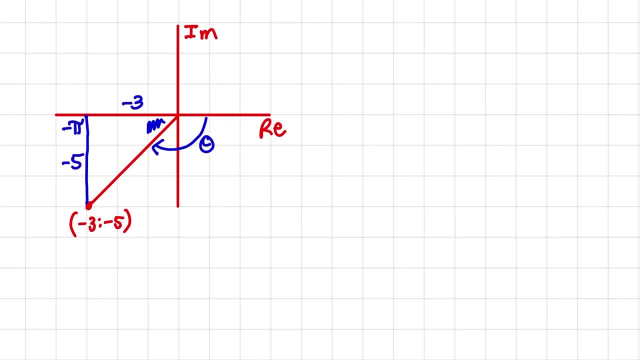 for the adjacent side and minus five for the opposite side. But, as in the previous video, we'll use absolute values. So, in order to find the argument of this complex number, I would consider negative pi, because I moved negative pi all the way back to the real axis, And then I'll add: